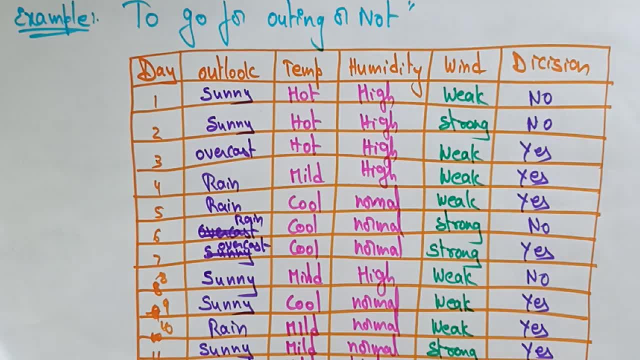 Hi students, welcome back. Now let's see the example of the decision tree learning. In the previous video I explained the algorithm. Now let's see the example on this Here. the concept is: I want to get one conclusion by seeing the weather, or whatever it may be. The thing is: 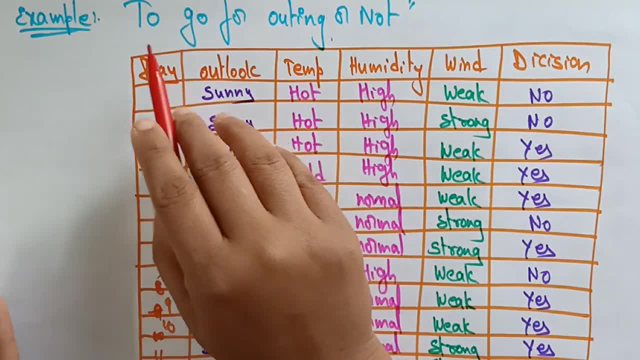 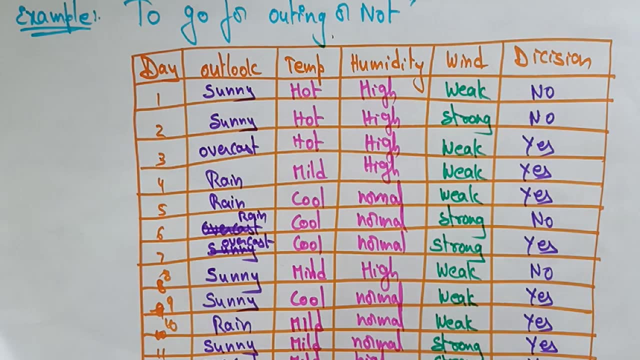 I want to go for outing, So the decision should be: either I have to go or not. Okay, yes or no. I need to be finalized So on which days I can go for the outing, on which case I'm not supposed to. 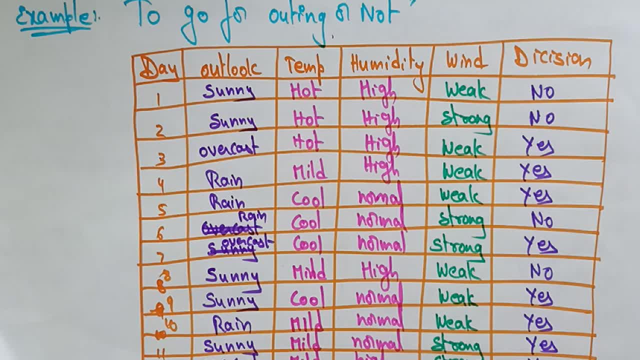 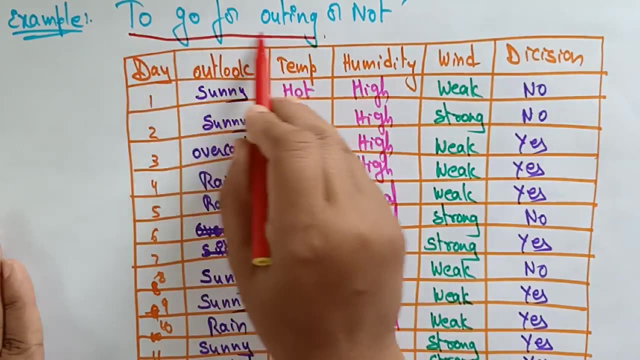 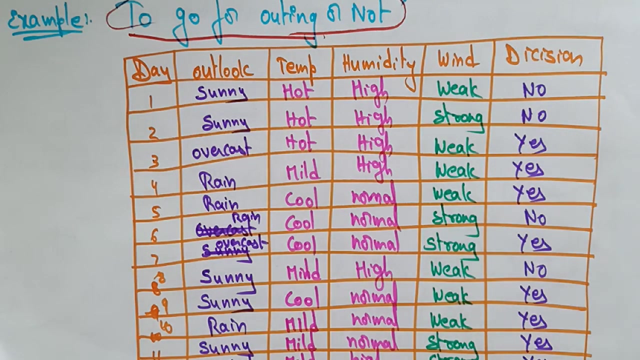 go out? Okay, so that will be depend on the weather forecasting. So how the weather forecasting people will be judged. identified by learning this observation. Okay, let's see. So the output is to go for outing or not. That I had to be verified. Okay, to go for outing or not? So here is some. 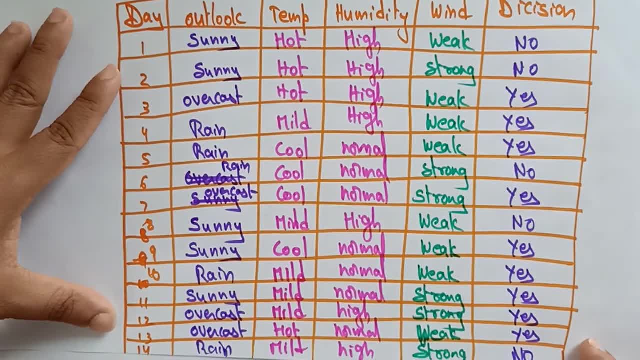 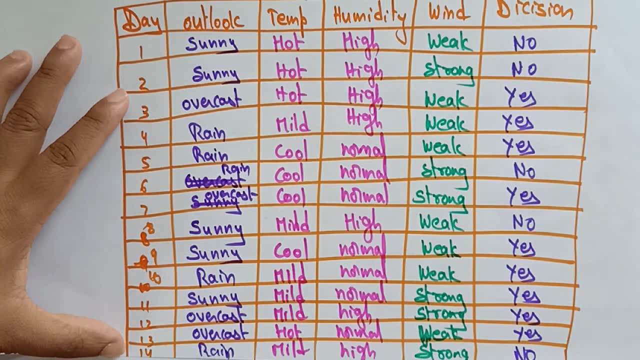 information they are given. So total: 14 days. I'm taken 1 to 14 days. In these days, in which day I can go for outing and which days I cannot go for outing, that I need to be find out. Okay, with the help of these attributes, Here they are. 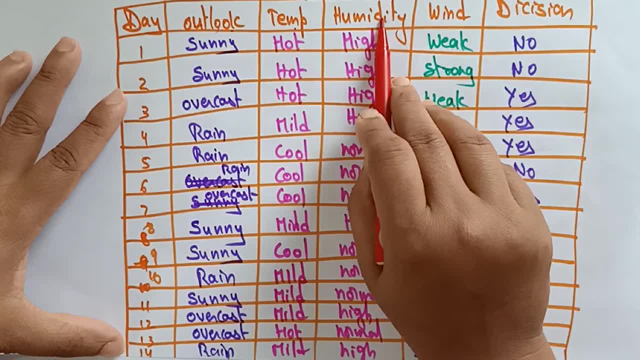 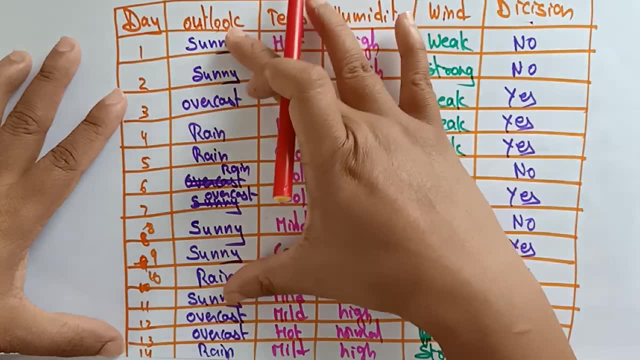 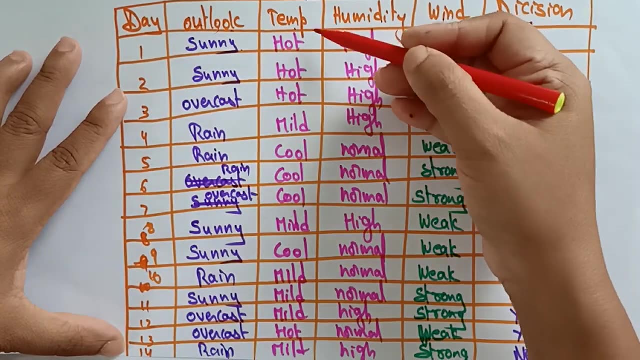 given attributes like outlook, temperature, humidity, wind and the decision. So the outlook is maybe sunny, rainy or forecast Okay. so for this output attribute, the nodes will be either rainy and the temperature should be hot, mild or cold, and the humidity may be high or a normal. 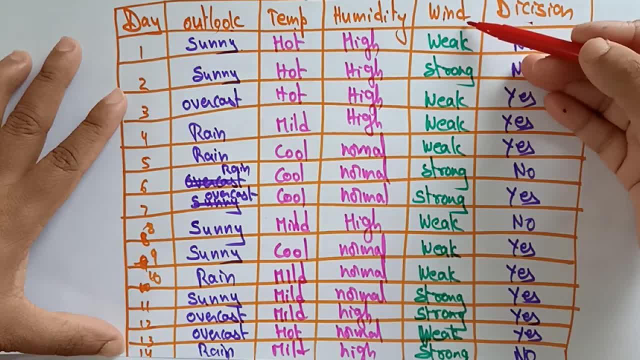 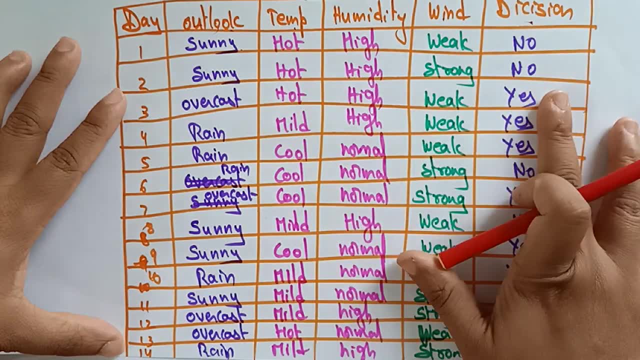 Some days it may be high and some days it may be normal, and the wind is. some days it will be weak, strong, weak strong, and decision is yes or no. So here only weak strong, yes or no, high and normal, and these two attributes is having sunny, overcast, rainy, hot, cool. 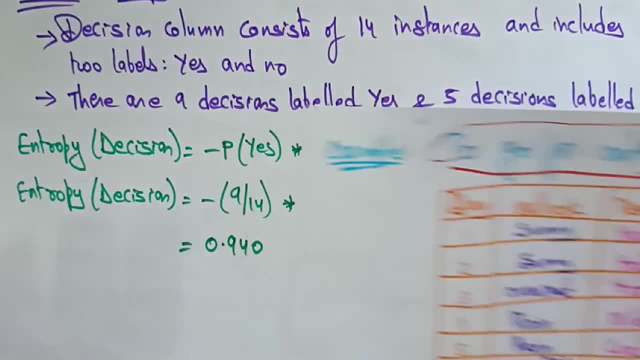 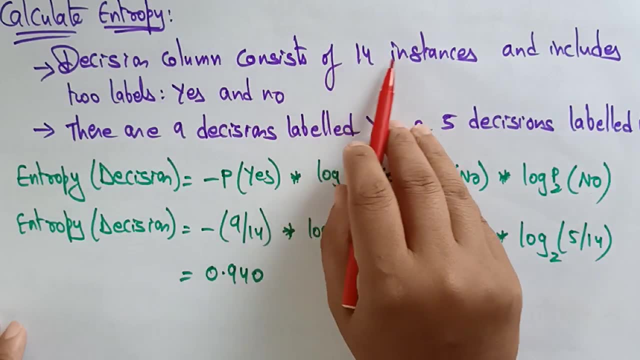 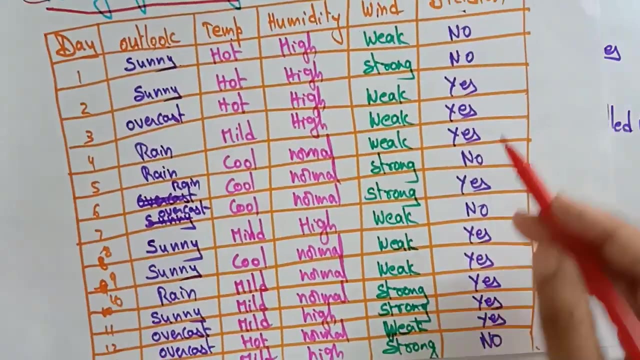 mild. So let's see the problem. First thing is you need to calculate the entropy value For the given problem. decision column consists of 14 instance. So here you can observe there are 14 instance and includes two labels: s and no. s and no, two labels are there, There are nine. 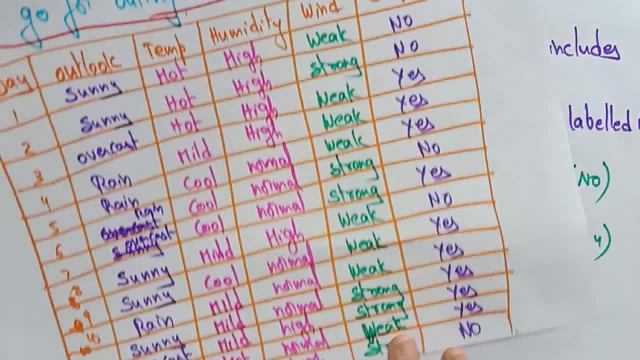 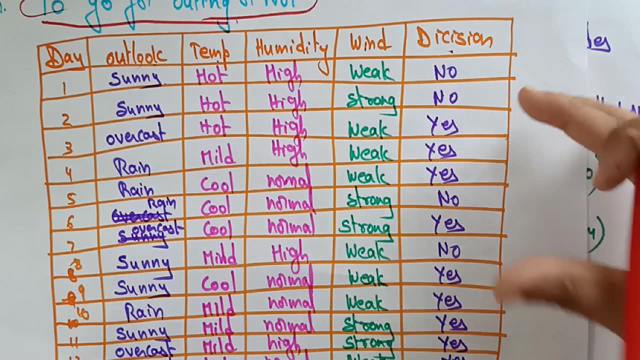 decisions labeled s and five decision labeled s. The first thing is you need to, you have to focus on decision, because I have to go outing s or no. So you have to calculate the entropy values with the help of decision and the attribute value. So you have to go outing s or no. So you have to. 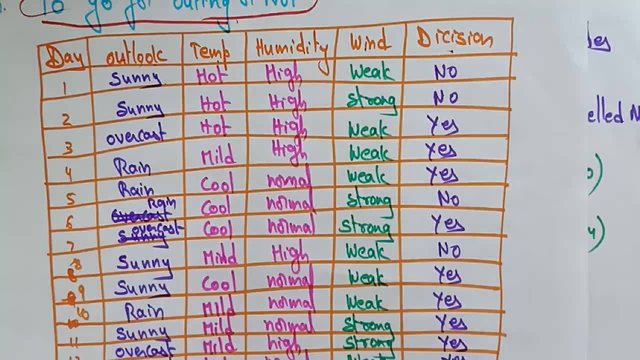 calculate the entropy values with the help of decision and the attribute value. So you have to do decision attribute, decision attribute, decision attribute, like that. So for each and every attribute you need to be calculate the entropy values as well as the gain value. So 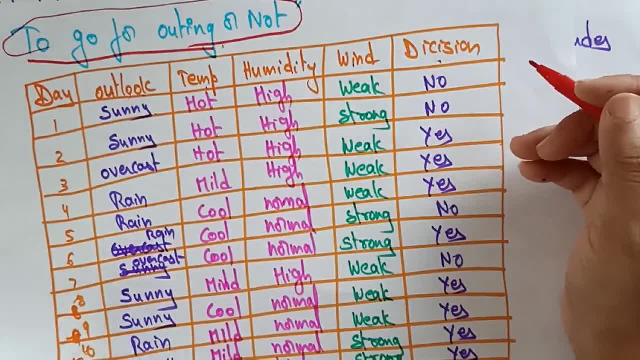 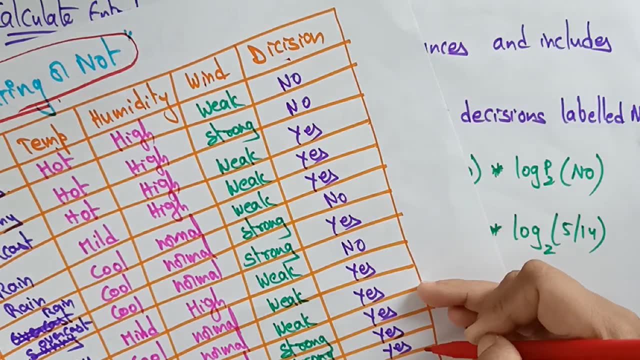 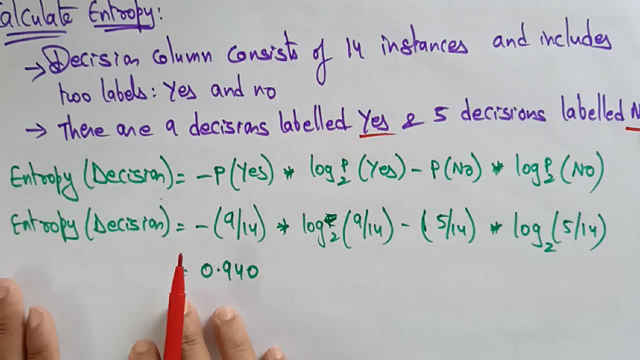 whatever I said in the algorithm. So, total, how many decisions yes will be there? Total: there are nine, nine decisions yes, one, two, three, four, five, six, seven, eight, nine decisions yes and five decisions are no. So the formula for decision: I am just calculating the entropy value for 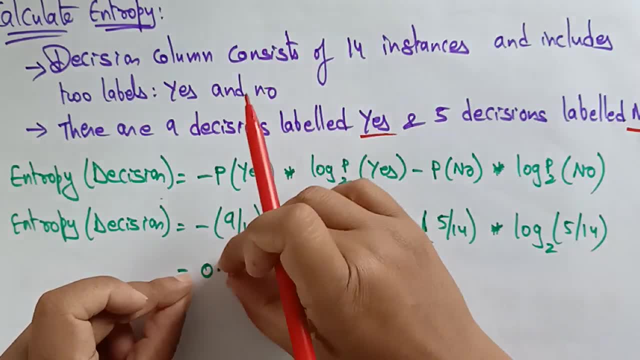 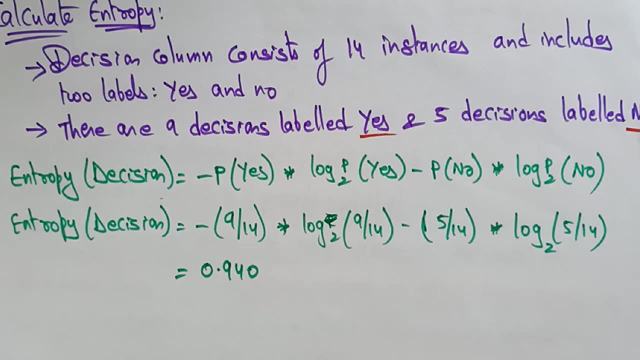 decision first. So whenever I calculate the entropy value, I am just calculating the entropy value for decision. I can put that value in when I compare with the other attributes like outlook, temperature, humidity. So for that the formula is: how many s are there, The entropy? 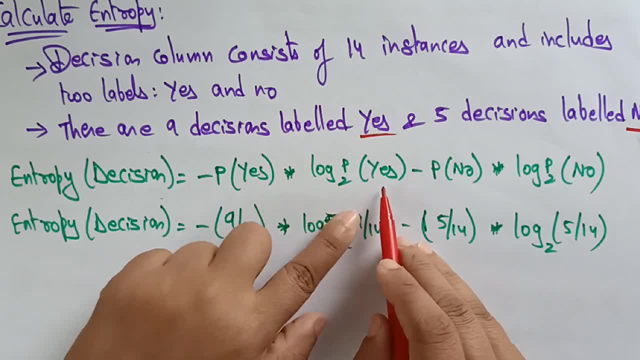 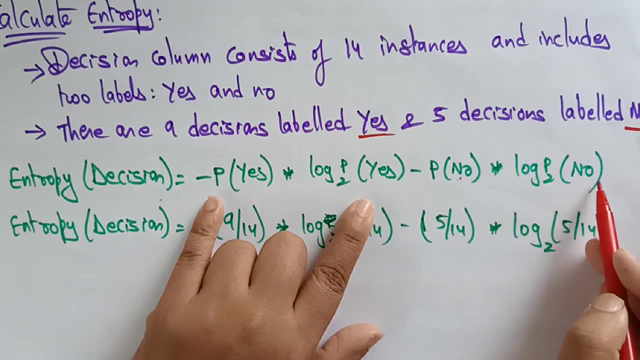 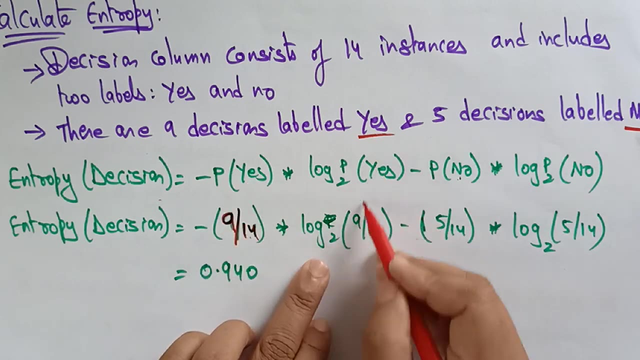 value s star. log p to the base 2 s and again the minus p. the decision is no log p to the base no, So just substitute. Yes means out of 14 days. nine days is yes Out of 14 days. nine days is yes Means in the place of p you need to write out of nine days. 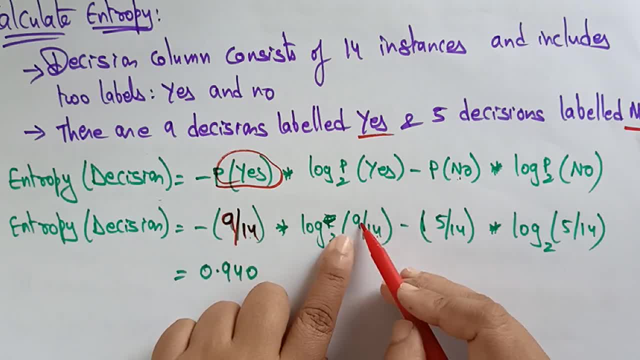 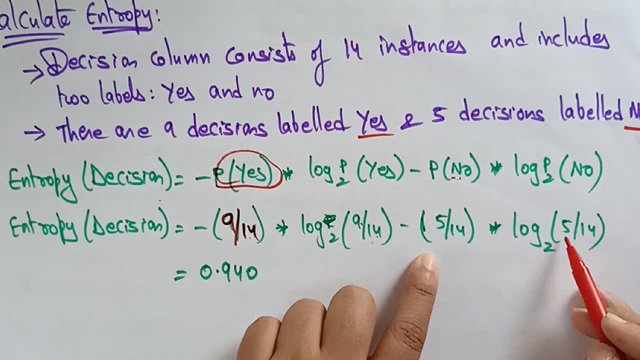 out of 14 days, nine days is yes. Out of 14 days, nine days is yes. In the same way, here: out of 14 days, nine days is f. five days is no. Out of 14 days, five days is no, Nine is yes. 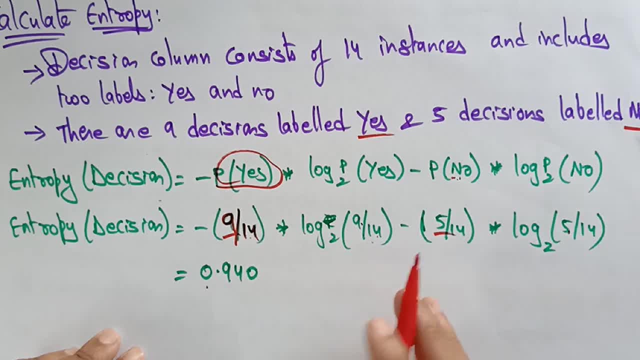 five is no. So if you, by using the calculator, you have to find these log values and the calculation, you will get the answer 0.940.. So this is the entropy value. So this is the decision. The entropy decision is 0.940.. Okay, So remember this. So what is the next step? 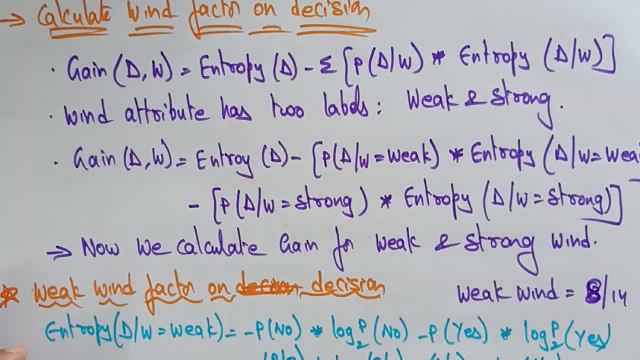 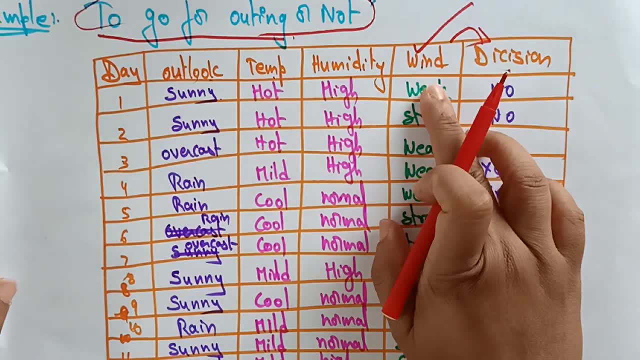 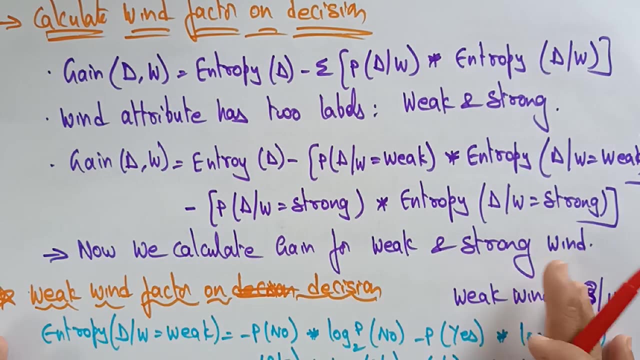 The next step is I need to calculate the wind factor on decision. So first I am taking wind, Let me take wind this attribute on decision. I am taking the wind factor on decision. So the gain for this, so entropy value for decision, I calculated. Now I want to calculate the. 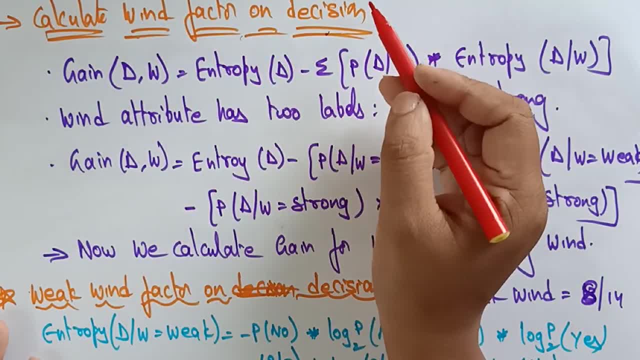 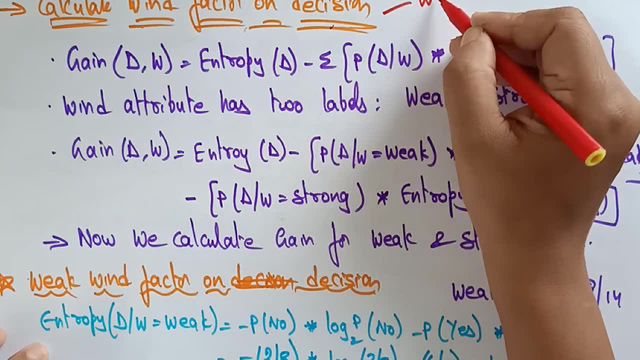 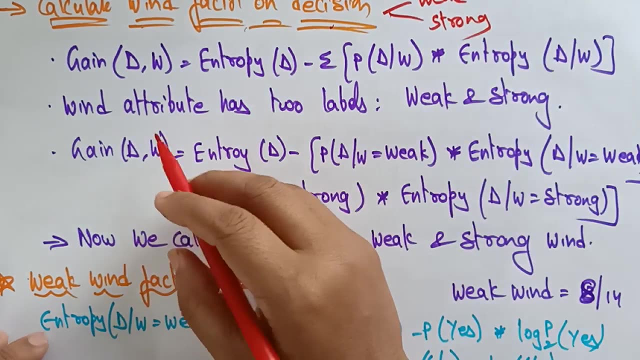 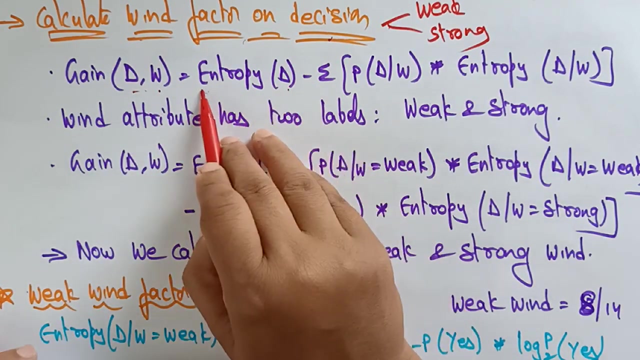 wind factor on decision. So here wind factor on decision is of two types, because the wind may be weak or a strong. So you need to calculate the wind factor: wind weak and wind strong factor. So the formula for here is: the gain of decision on wind is entropy of d, whatever the entropy of d that you calculated. 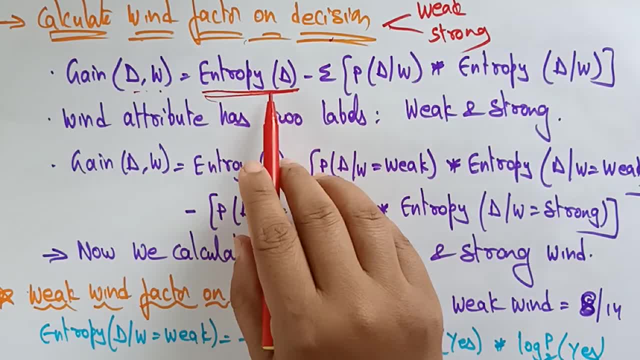 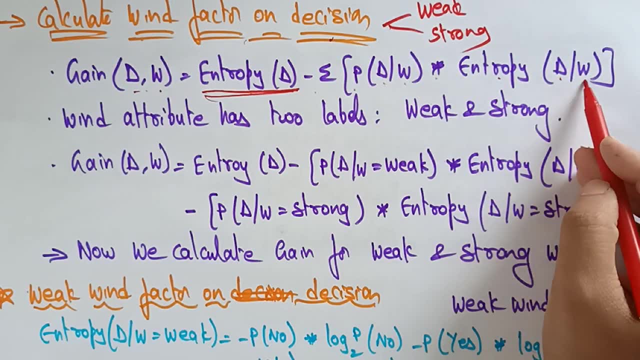 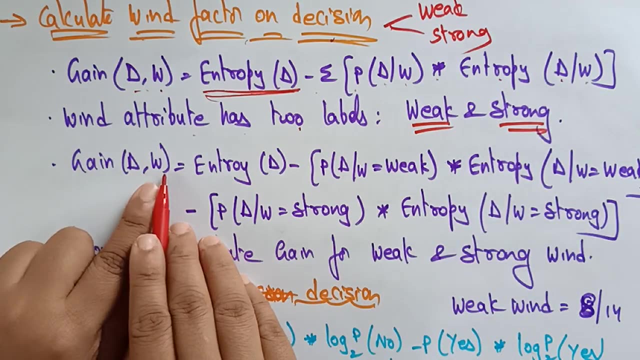 Okay, Just know the entropy value that you calculated, The entropy of d minus sigma of p. decision on wind. star entropy decision on wind. Okay, So the wind attribute has two labels, weak and strong. Okay, So the gain again substitute. here I am splitting this formula into two. 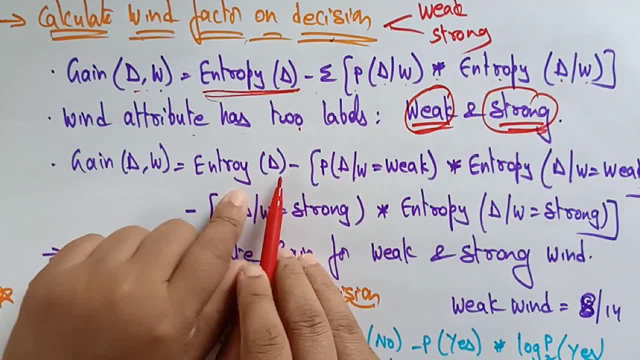 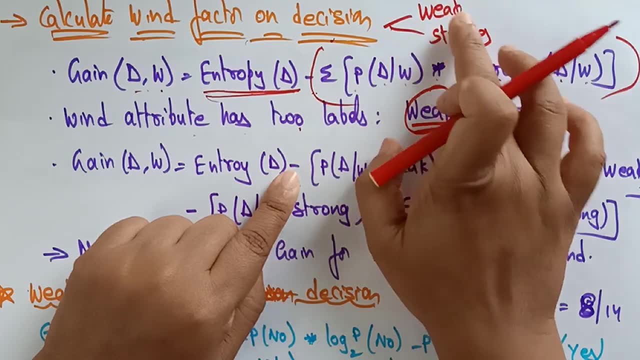 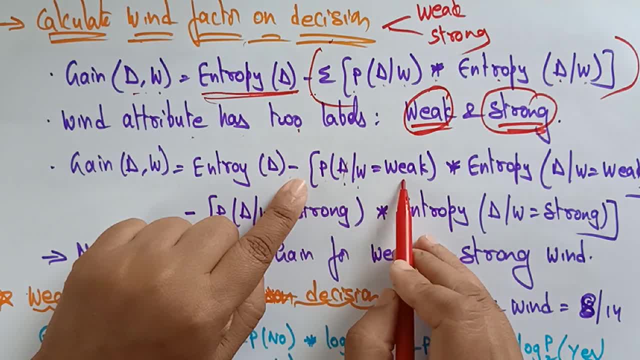 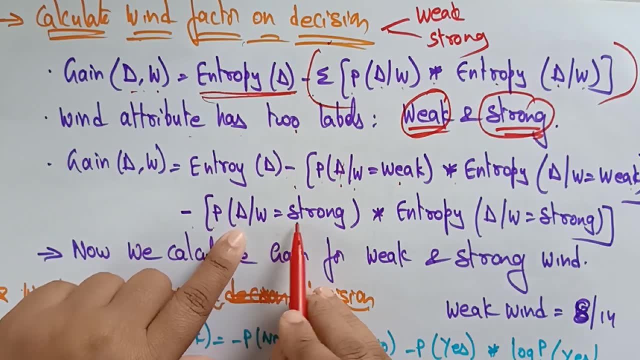 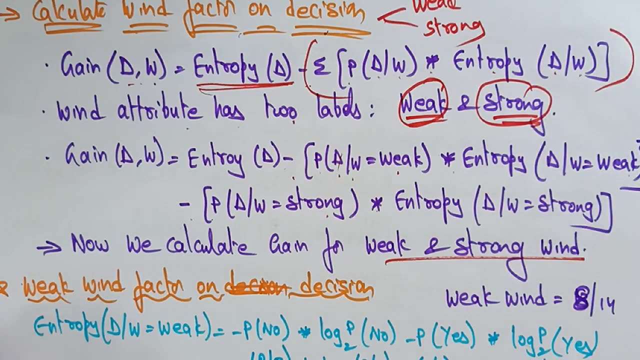 I am taking p decision of wind is weak into entropy of decision of wind is weak. minus again p decision of wind is strong into entropy of decision of wind is strong. Now we calculate gain for weak as well as the strong. Okay, So apply this, So substitute the values is So first, 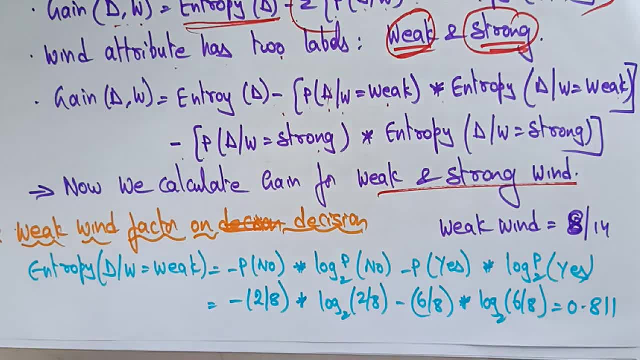 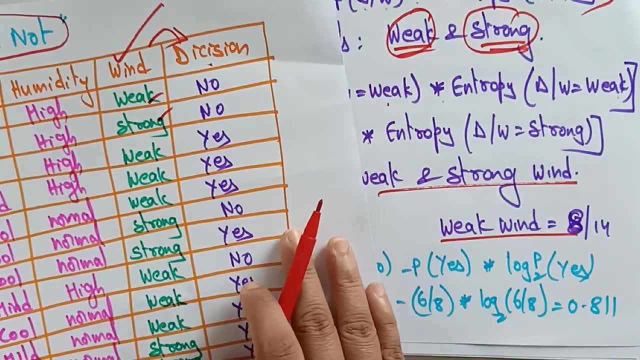 thing is: how many in the weak? how many decision is yes and how many yours no. Okay, The weak first. calculate the weak wind In the weak wind. let's take the weak wind, So how many are? no One In the weak? 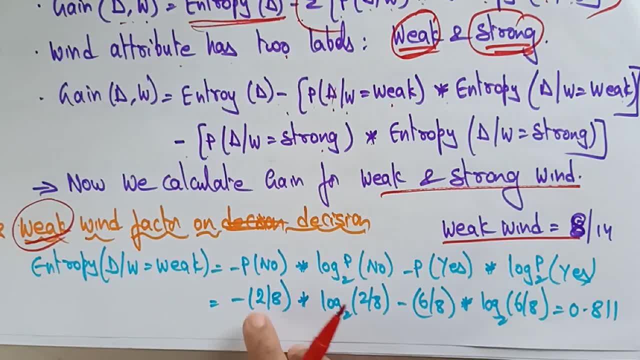 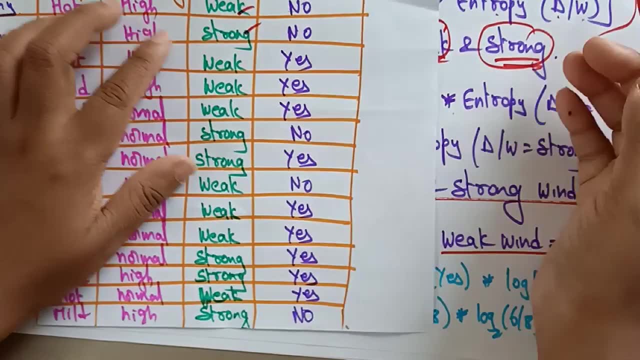 wind. two, Okay, Only two are no, Only no is two. So in the strong, how many yes are there? I have to talk about only the weak wind. which one is having no and which one is having the S? Okay? 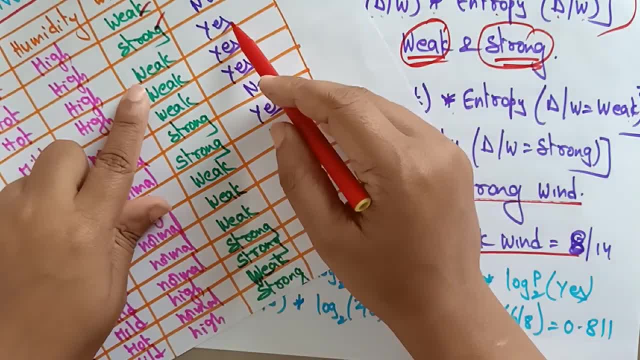 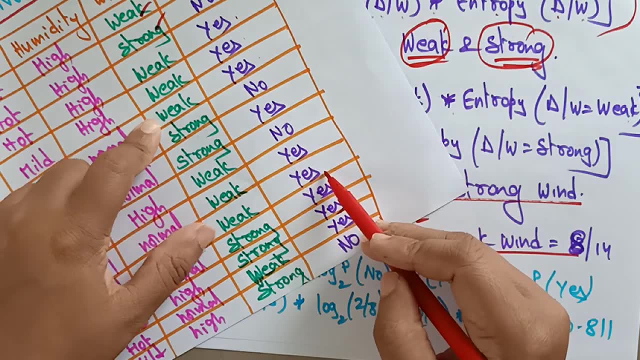 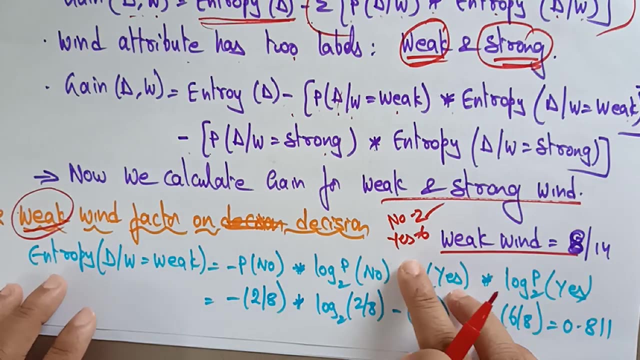 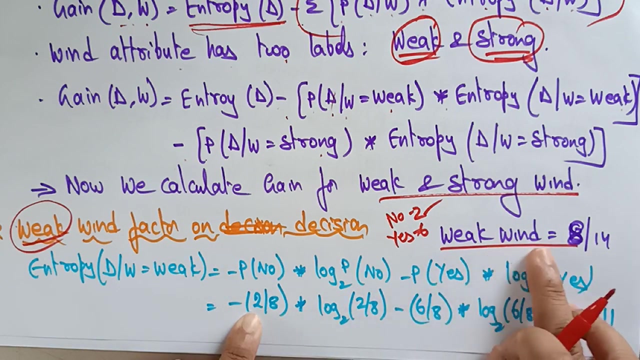 So the S is: let's see how many yes are there in a weak weak wind? Yes, one, two, three, four, five, six. So six are in a weak wind. the decision for no is two and decision for S is six, only for the weak wind. So I substitute here. So total weak winds are: 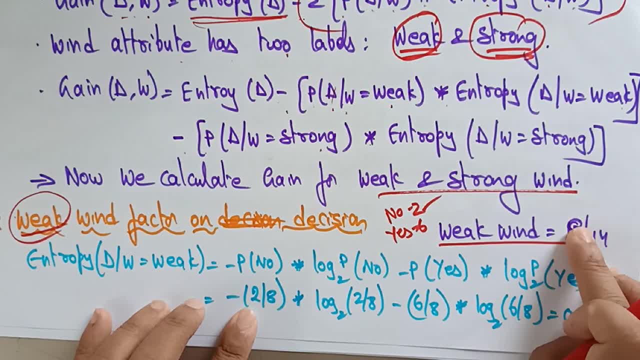 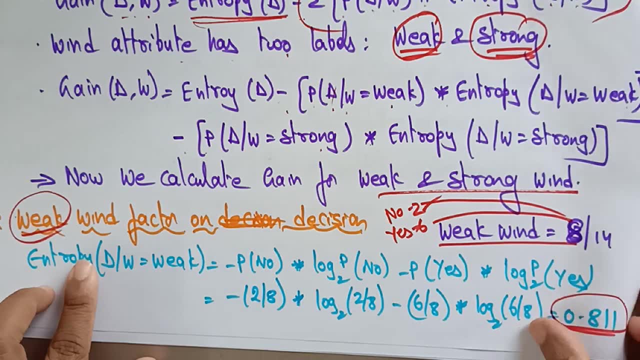 total, eight are there Out of 14,. eight is a weak wind. In this eight, two are no and six are yes. So substitute here and you will get this answer. This is only for weak wind. In the same way, you need to calculate for the strong wind factor. 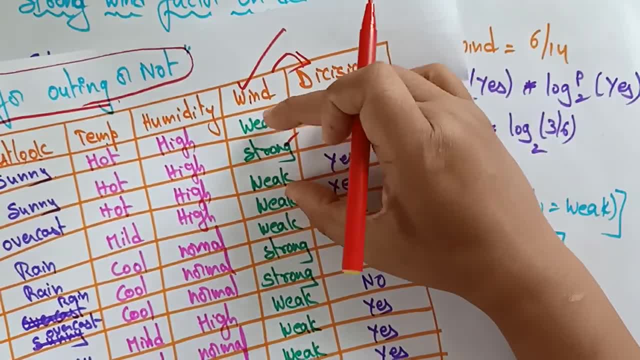 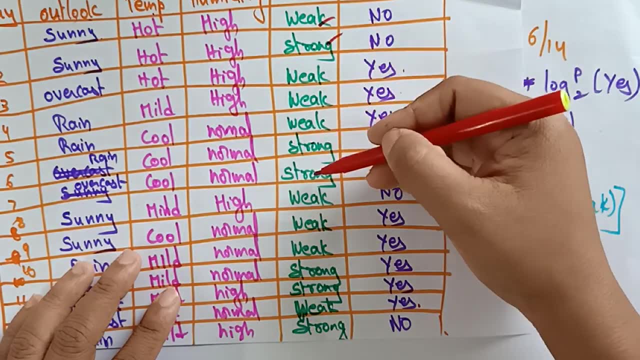 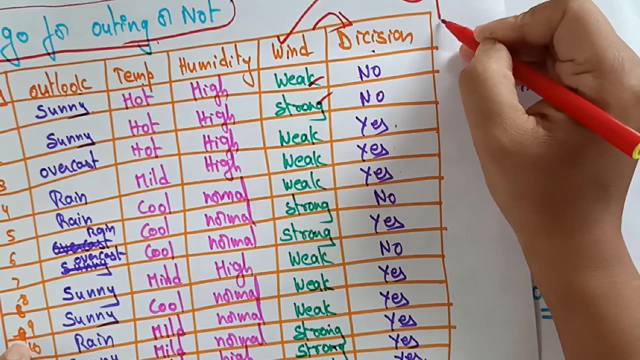 So we are calculating only this wind. So first calculate the decision on weak, now coming to the strong. So here, how many strong winds are there? One, two, three, four, five, six, Total six strong winds are there. So out of six strong winds, how many are decision? 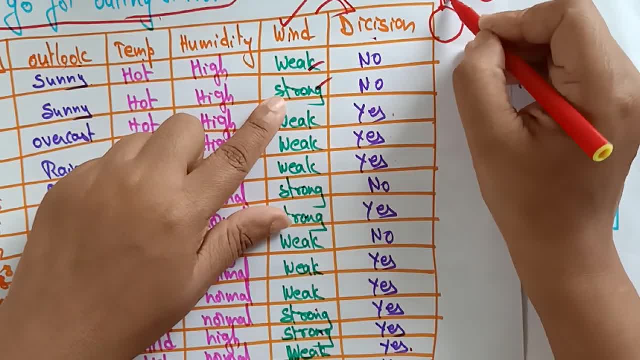 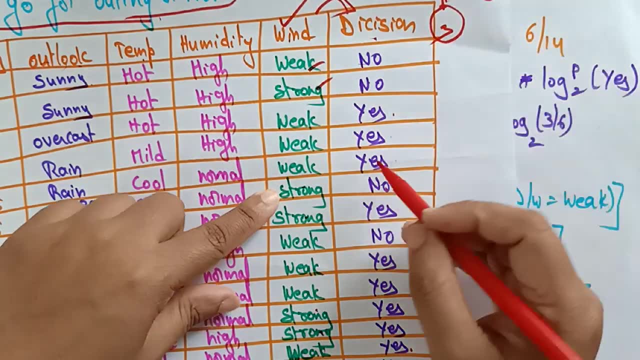 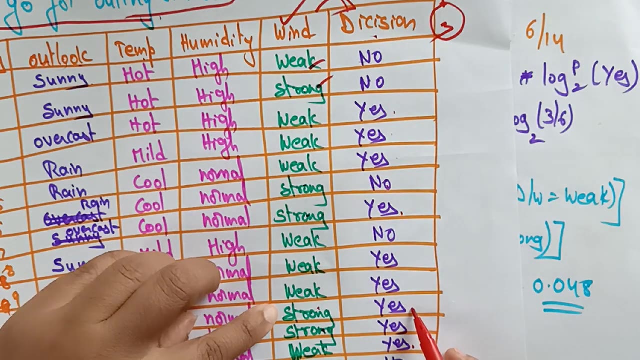 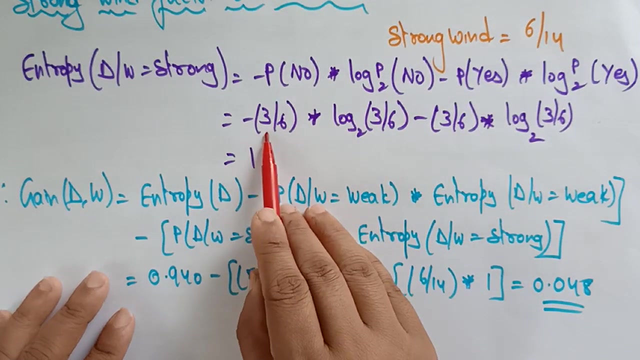 yes. and how many are decisions? no, Let's take no. How many decisions are no? One, two, three, Three are no and S C Yes. we had to see So strong. where is strong? S? One, two, three. So out of six, three is no and three is yes, So substitute here: Three is no. 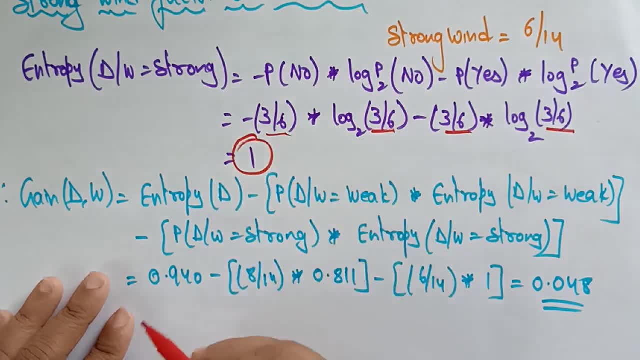 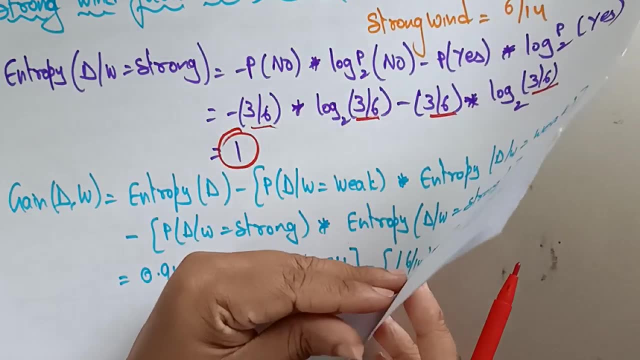 and three is yes, You will get the value of one. So after you are getting the entropy values of weak wind and strong wind and substitute that values in this formula. So just now, whatever you calculated, So this is a formula okay for weak wind and the strong wind. So 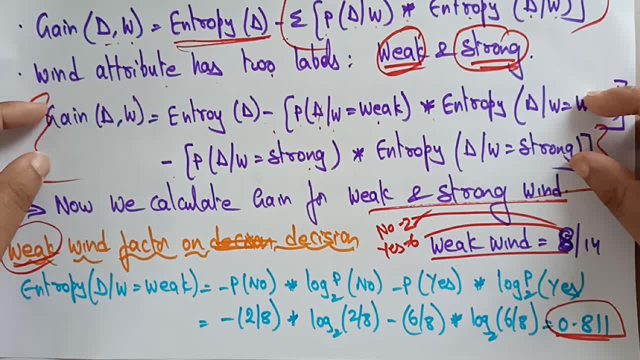 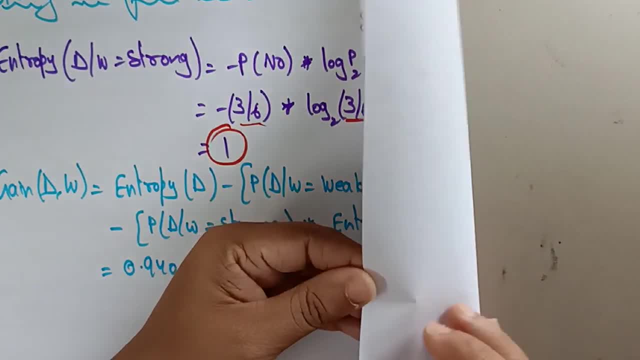 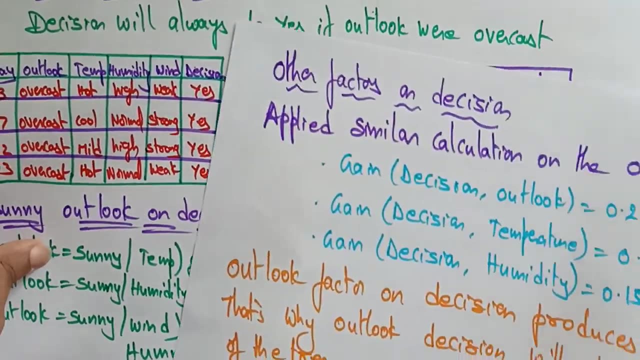 substitute the values in this formula, you will get the gain value. So whenever I substitute the values, I will get the answer as 0.048.. So this is the gain value for the strong as well as the weak wind. So let me calculate the decision on outlook temperatures also for this. 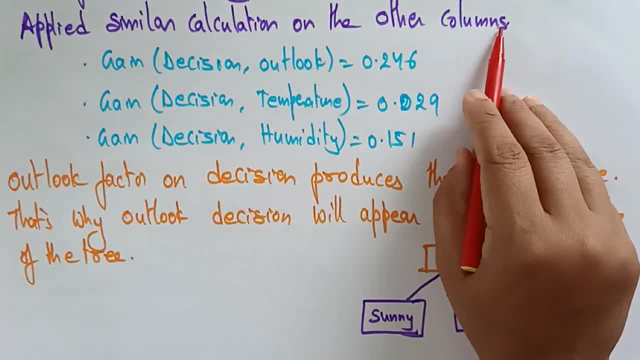 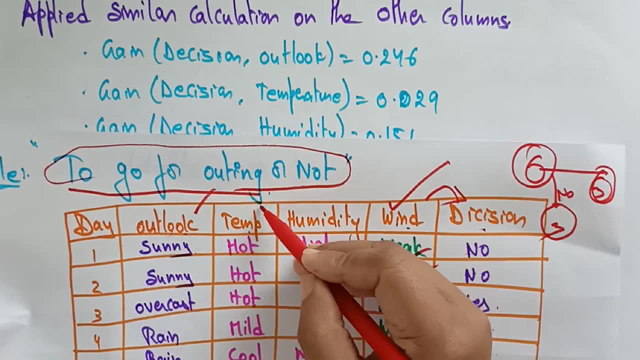 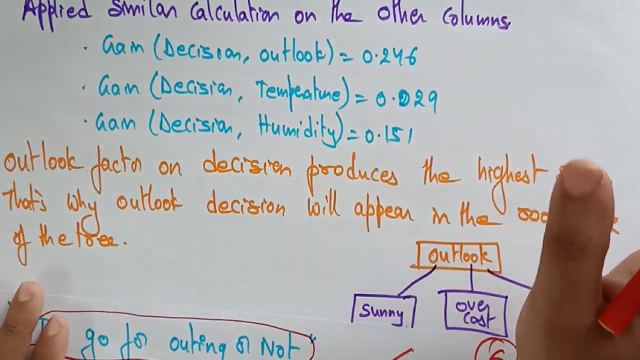 The other factors on decisions applied similar calculation on other columns like: So whatever the applied here in wind, you just applied the same method: outlook, temperature and humidity also. So after that you will get these values. In these all values, you need to check which one. 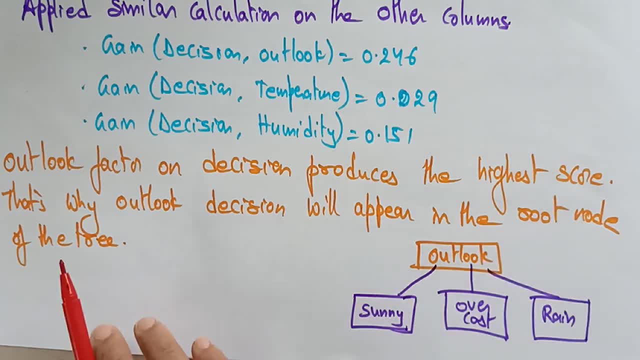 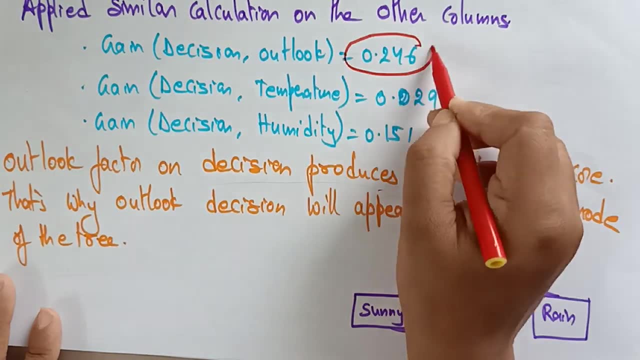 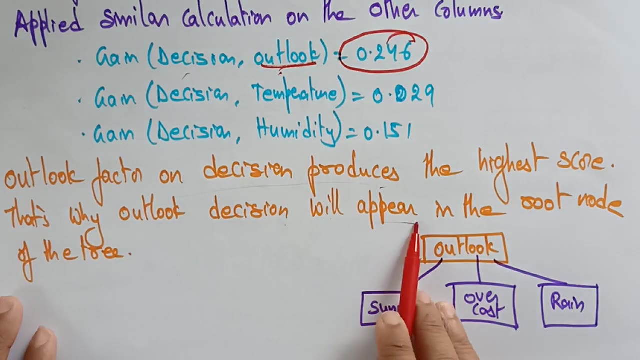 is having the highest value. Okay, that you have to be taken as the starting node. The outlook factor on decision procedure is the highest value, So this decision- outlook- is having the highest score. That's why outlook decision will appear in the root node. 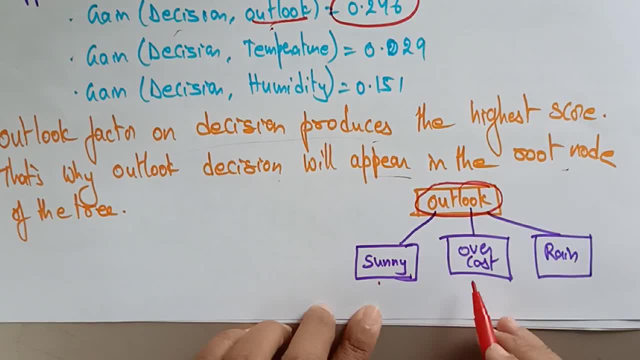 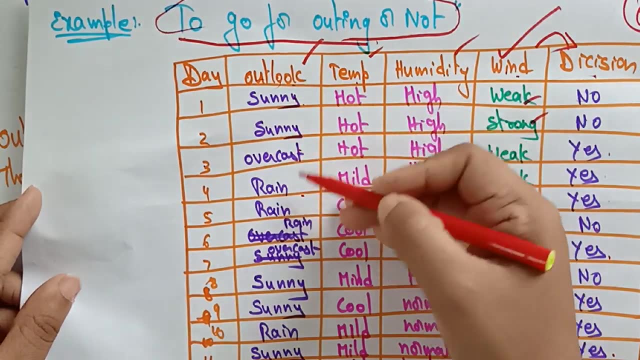 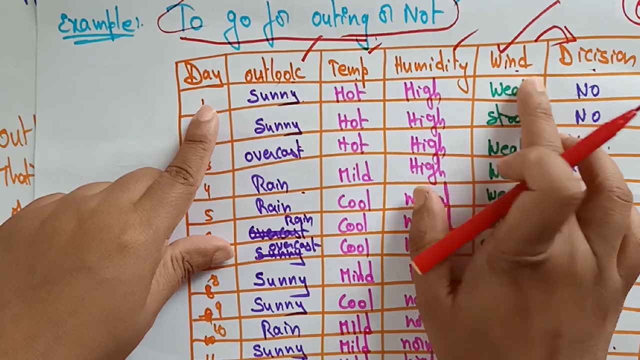 So here it is: appears in the root node and the sunny. So what are the attributes in the outlook that the notes of the outlook is sunny, overcast, rain means. in all these 1234, in all these four attributes, We need to find out one as a selection because we can't observe everything. 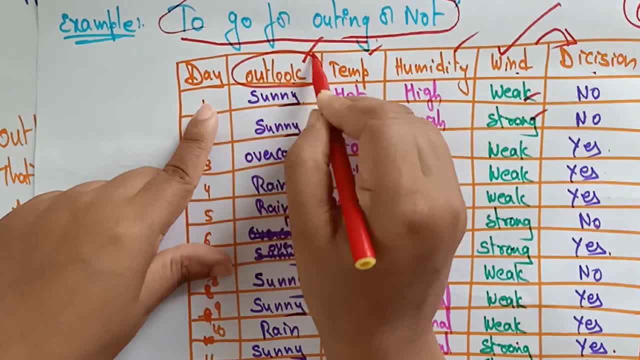 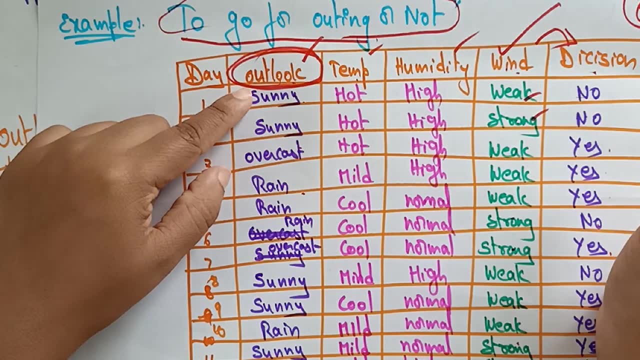 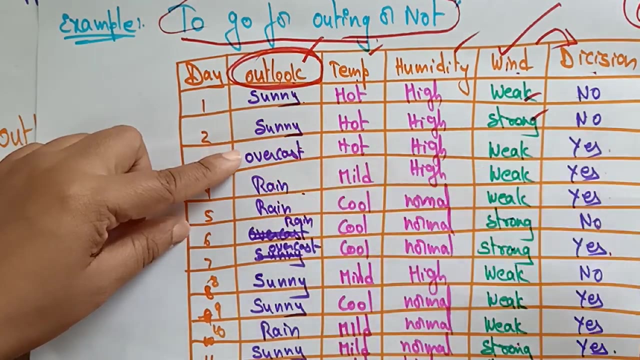 so in all these four, i had taken a decision on outlook. by calculating the entropy and the gain value, i found this is: this is getting the highest value. so now i'll i'll just observe outlook. so in sunny, what will be the decision? if it is overcast, what will be the decision? if it is rainy, what will? 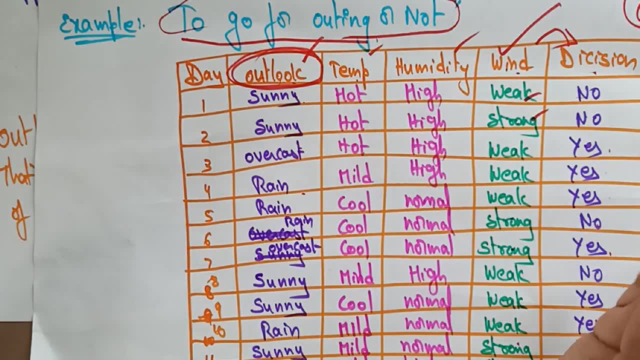 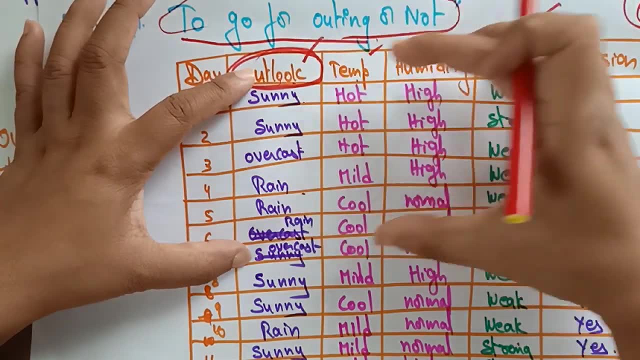 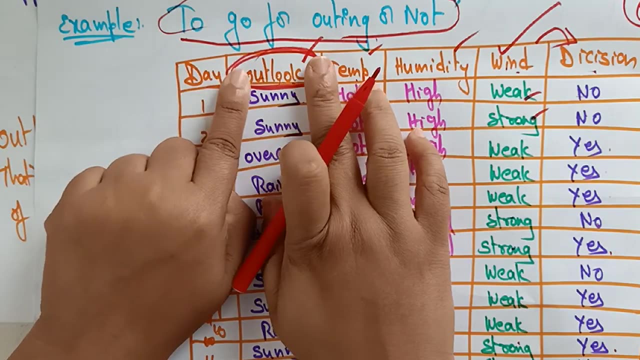 be the decision on which days it is sunny, on which days it is overcast, on in which days it is rainy, so when i can go and when i can't go. so everything i it's based on the outlook. so i'm just discarding all these things, three things, because outlook is get the highest point. so i'm just taking this as 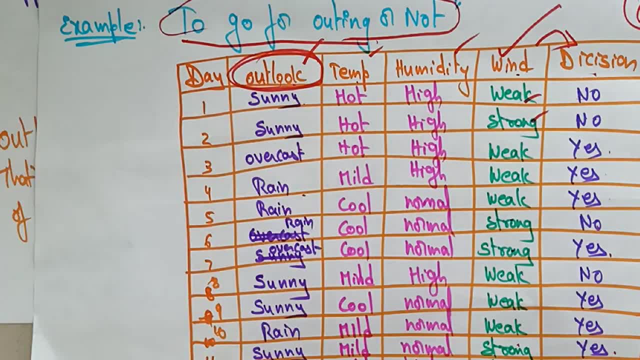 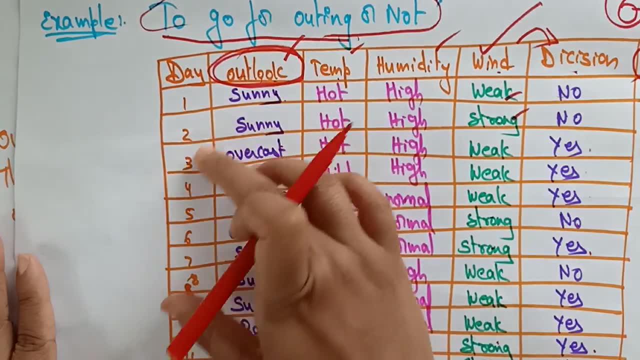 my root node and i'm working on this. okay, the first thing is, whatever the attributes they are given, you have to first find out which attribute becomes the root node and that the sub nodes are all the nodes that are present here, sunny or whatever that nodes that are present on that. 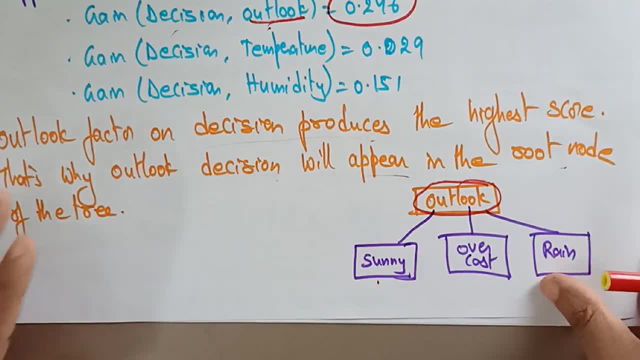 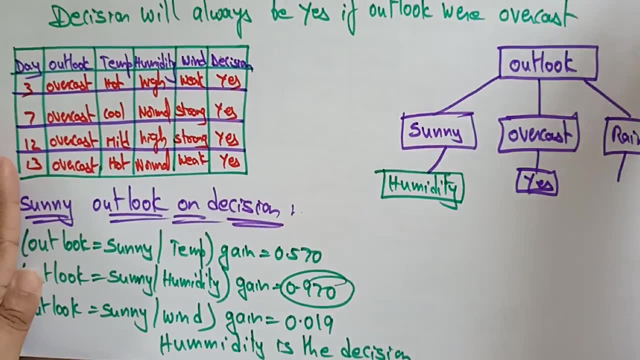 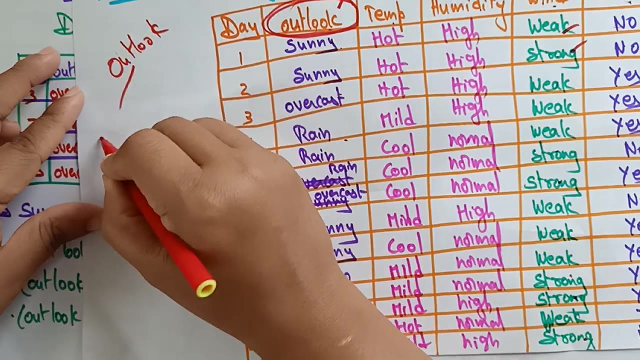 attribute. okay, so discard the temperature, humidity, wind, everything and focus on the outlook. so now overcast outlook on this. so here in the outlook you are having three parts. right in the outlook you are having three parts. one is the sunny and one is the overcast and another is. 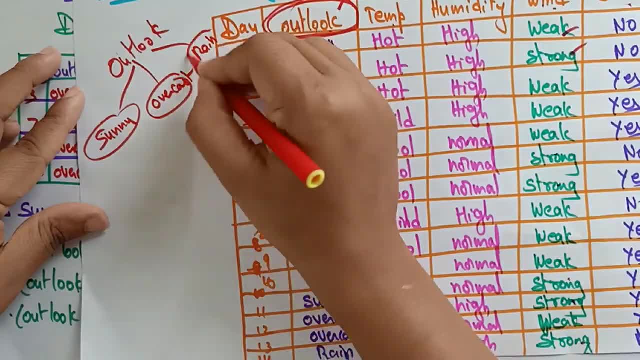 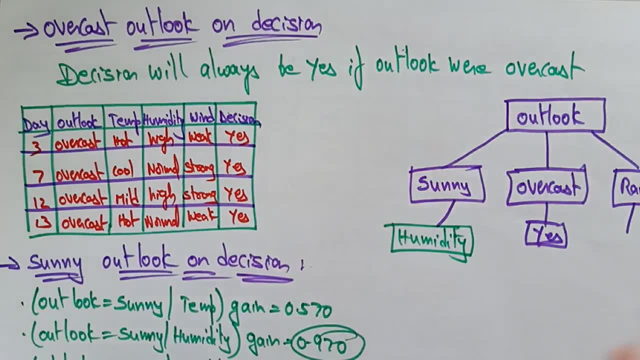 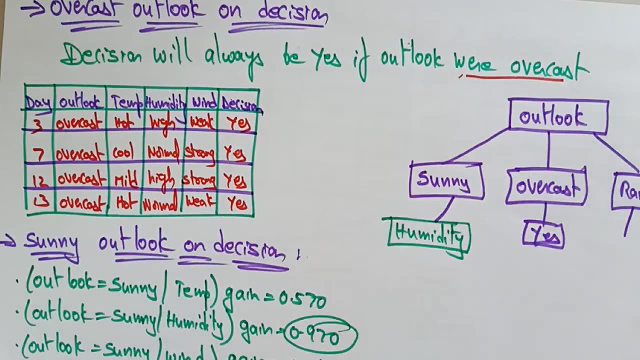 the rain. so again, in all these three things, you have to find out the decision. the first: let me take the overcast outlook on decision. so first, let me take on overcast on decision. the decision will always be yes if outlook were overcast. so if you take this overcast wherever the overcast is there, the 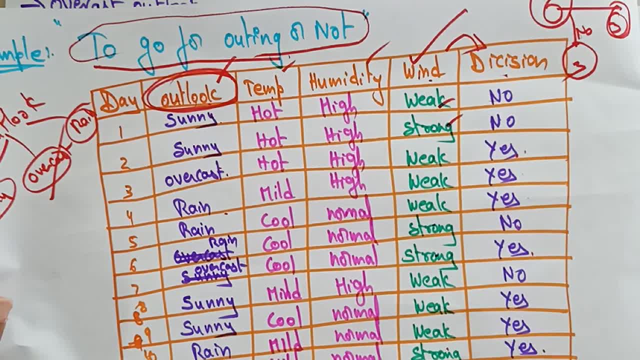 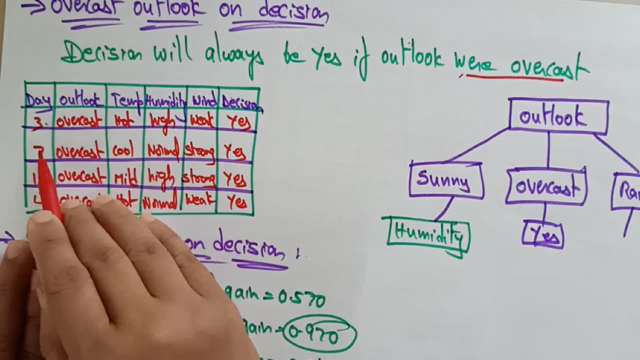 decision is: yes, overcast, yes, overcast, yes, okay, overcast, yes. so there is no need to find out any formula, because where in the day 3, day 7, day 12, day 13, outlook is a overcast and the temperature is hot, cold, so don't forget, overcast is a overcast, so, don't forget, overcast is a overcast, so don't. 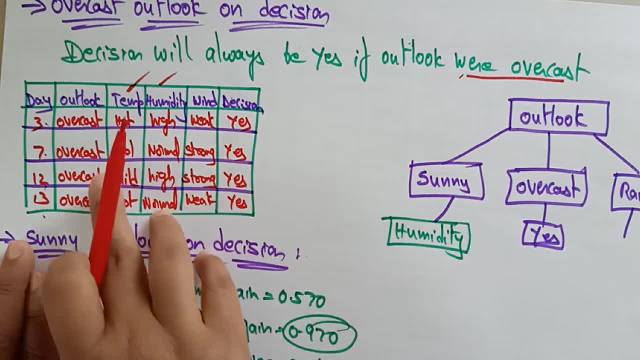 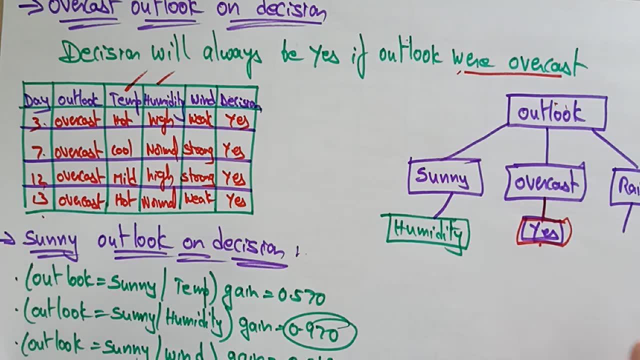 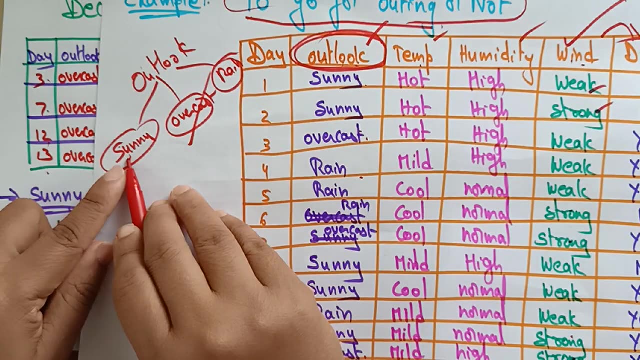 forget about temperature, humidity and wind, whatever it may be thus, but the decision is yes, so directly, keep on under the overcast. it is yes, so overcast is over. now let's calculate the sunny outlook on. decision means focus on this sun, so sunny may be the hot, or whether it may be a hot. 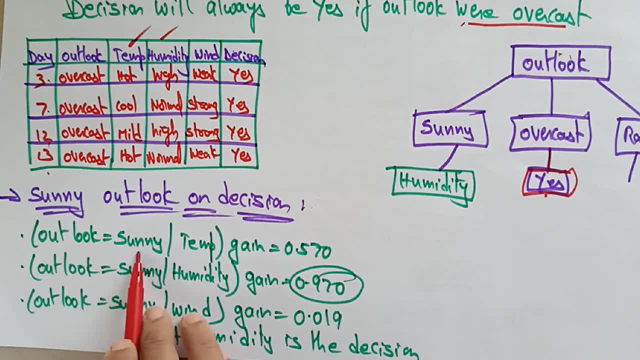 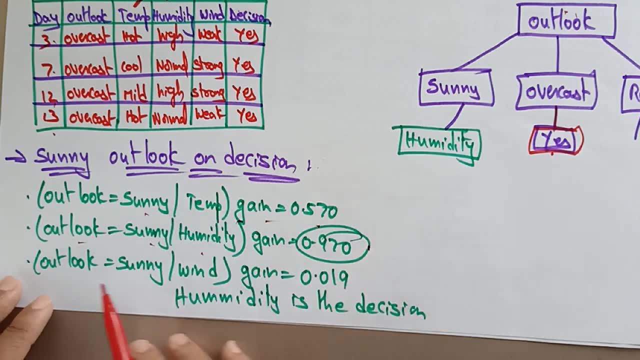 or mild or whatever it may be. so let's see the outlook sunny. on temperature gain calculated. so outlook: sunny. if it is a humidity temperature, it is a hot or mild or whatever it may be. so let's take humidity, you need to calculate the gain value, the outlook. if it's sunny, it is a wind, you need to. 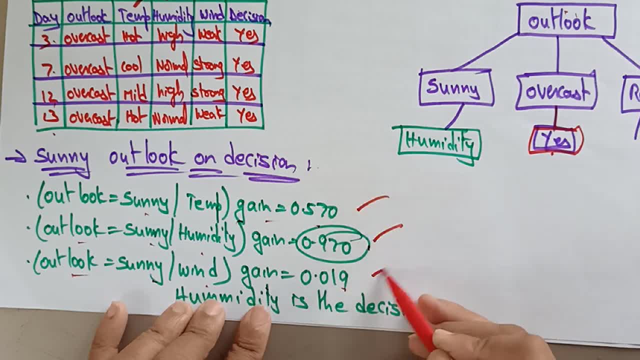 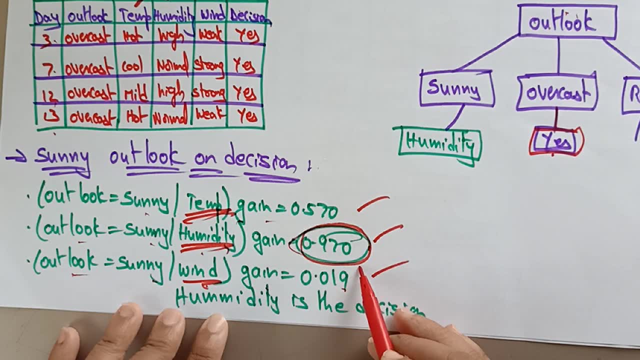 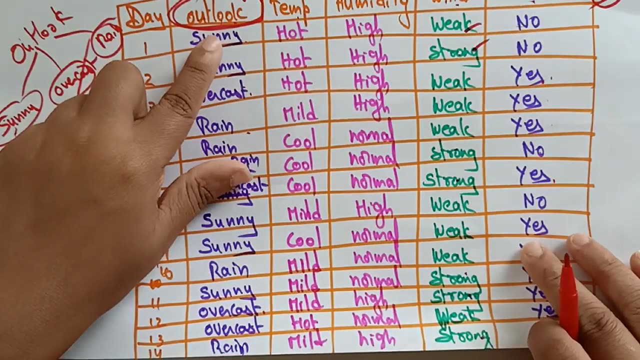 calculate the gain value. so for all these outlooks, you need to calculate the gain value for temp on temperature, humidity and wind by all these things, 0.970. highest value, that is humidity, is the decision. for the sun, you have to consider the humidity. for sunny, you have to consider the 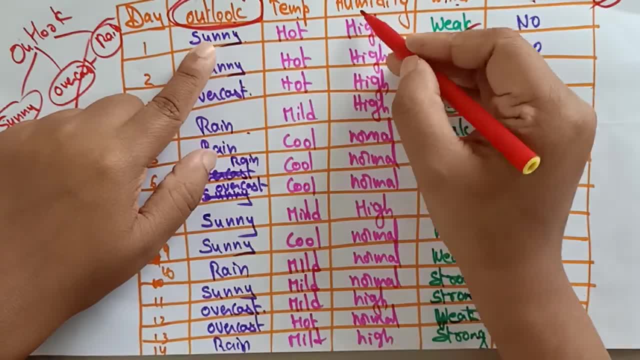 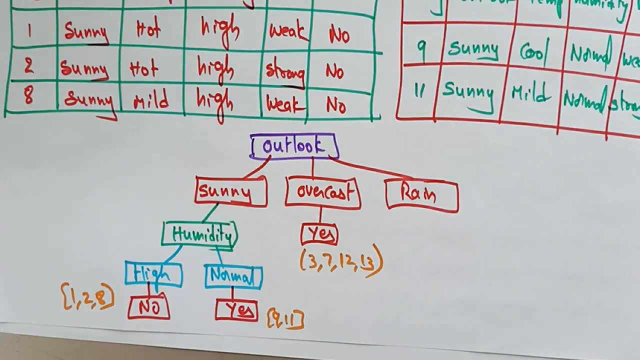 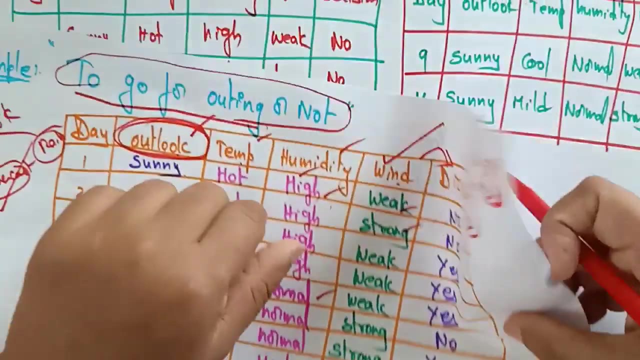 humidity: also okay for sunny. you have to take humidity, okay. so next, check if humidity is high or normal, because here there are two options, are there, because sunny is focusing on the humidity. so here two options are there: high or normal. okay, so what is the decision, what we had to take? suppose, if the sunny outlook is, uh, sunny, you have. 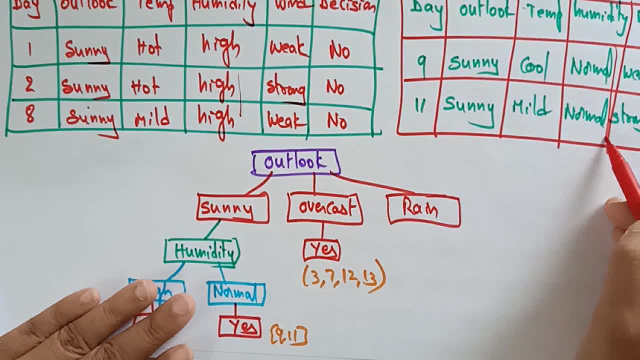 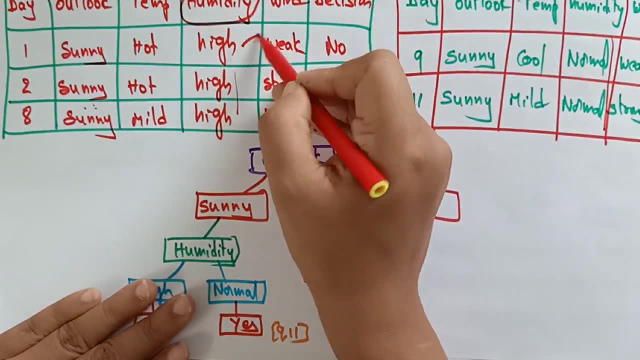 taken all the high in one and all the normal in one. okay, the one, two, eight days. those are the sunny outlooks and the humidity. i have to focus on humidity. the humidity is high, high, high, and here the humidity is normal, normal, normal. so wherever the humidity is high, the decision is: 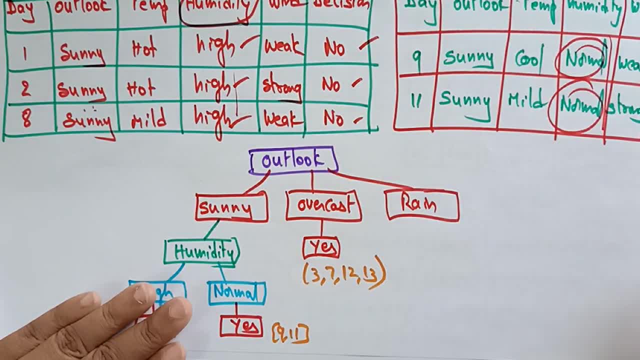 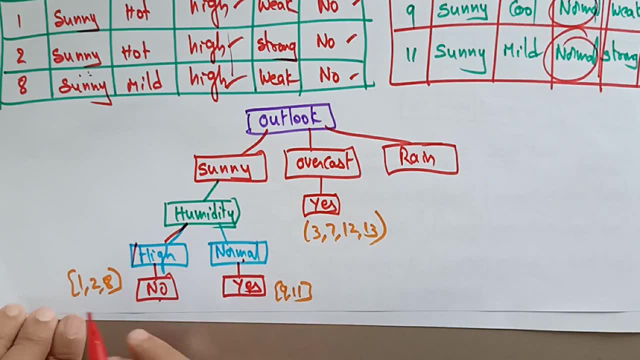 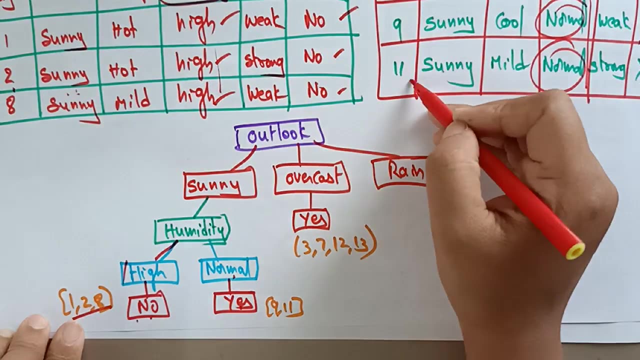 no, no, no. and wherever the humidity is normal, the decision is yes. so just keep humidity on high. it is no, the humidity on normal, it is yes. so on which days? it is no: one, two, eight days, it is no means. in those days i am not supposed to go out. in which days it is yes, 9, 11. so in the 9- 11 days i can go. 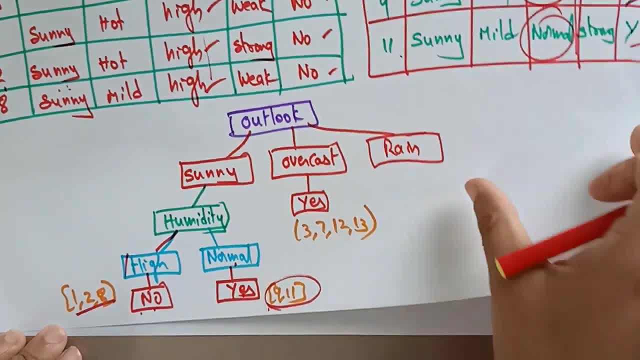 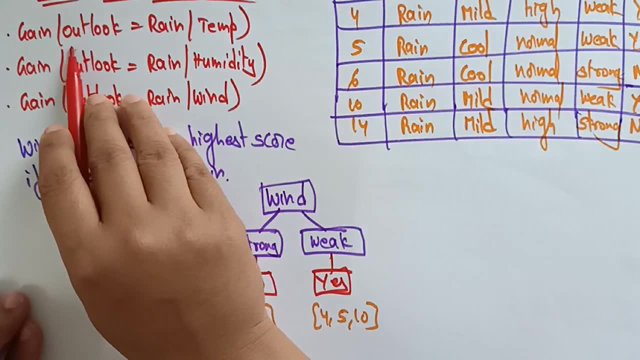 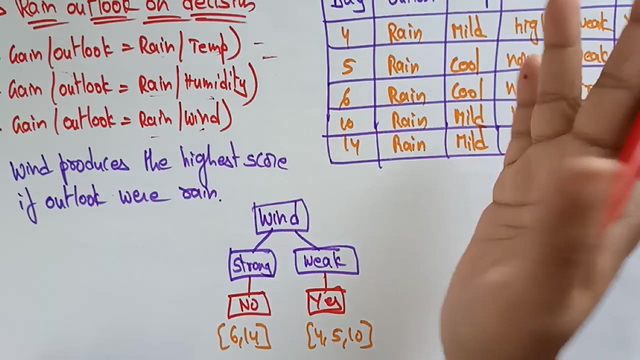 out. okay, so in the same way for calculate for the regulation also, the rain outlook on decision, so you have to calculate the gain outlook for the rain on temperature, rain on humidity and rain on wind. okay, you'll get some answers, so otherwise you just observe here. so i'm just taking the rain wherever i got. so in these days, where, whatever the rain, 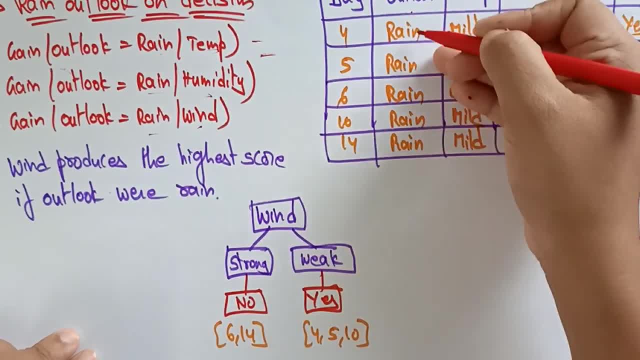 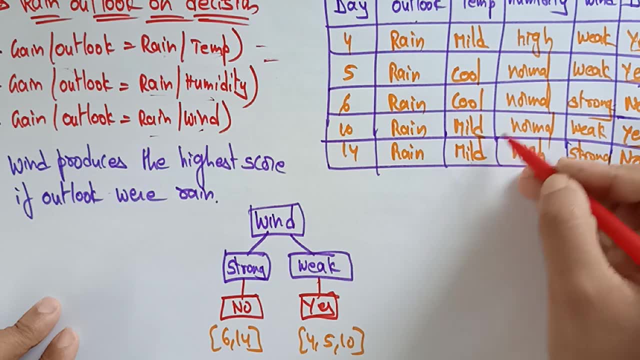 days are there. i just know down here, four, five, six, ten, fourteen are the days where the rain outlook is there. so, uh, on those days, the temperature is sometimes mild, cool, cool, mild, and humidity is like this, wind is like this, decisions are like this. okay, i'm taking wind. 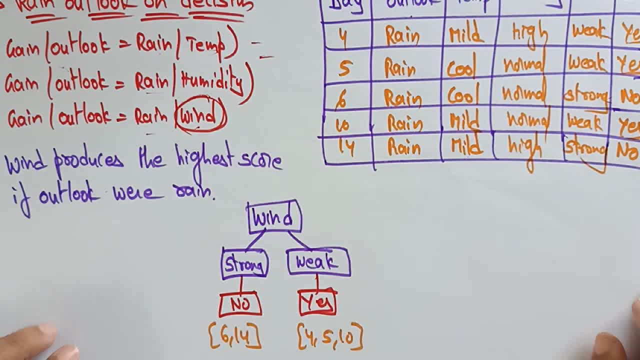 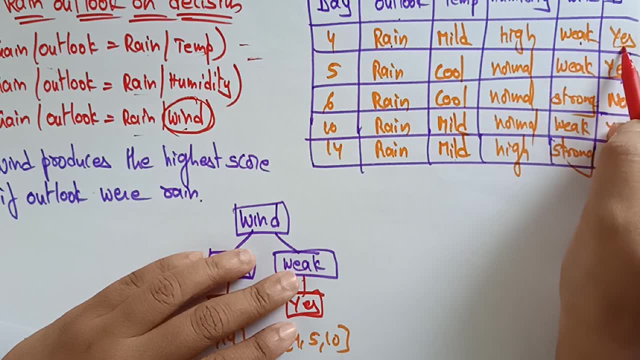 produce the highest to score. how can i say the wind produce the highest to score? let's see so: the wind. wherever the rain is there, wind is weak and decision is yes. wherever the rain is there, the wind is weak. decision is yes, okay. wherever the rain is there, wind is weak. the 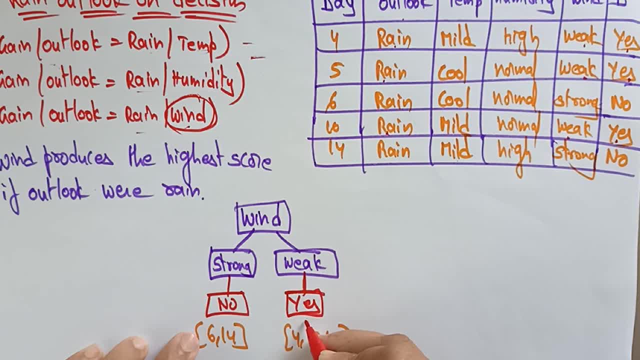 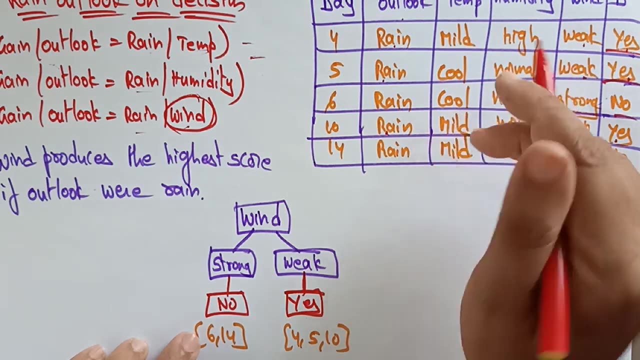 means obviously the weak becomes yes and the strong comes no. so here there is no conflict. there is one clarity some: wherever the weak wind is there, we are, we can go out. wherever the strong wind is there, we are not supposed to go out. but if you consider the other things, suppose if the rain, uh, if you take the humidity, let's take humidity. 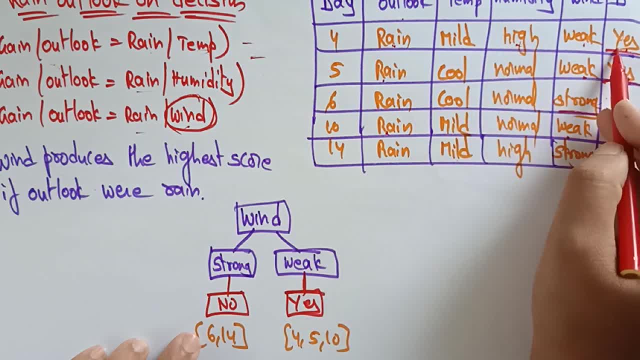 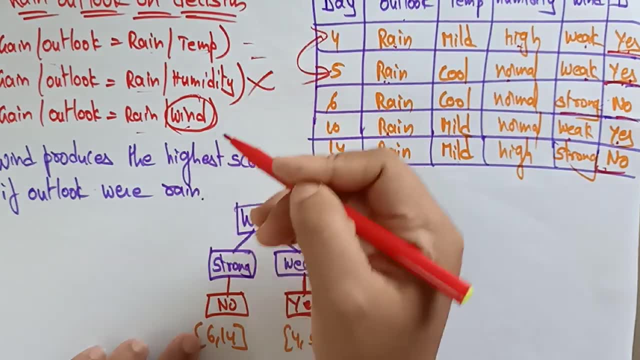 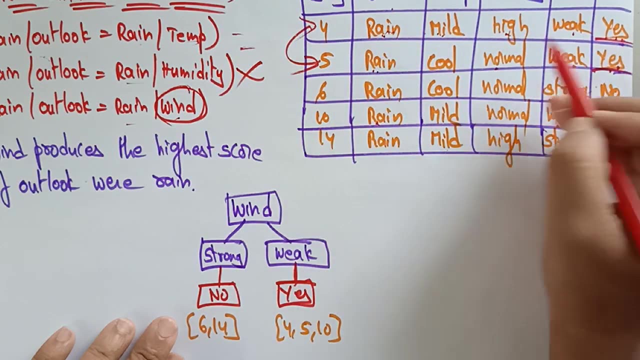 if rain is there, humidity is high. it is yes. if rain is there, humidity is normal. again it is yes. means some conflicts is getting here, so just discard it. if you just take the temperature also, whenever the rain is mild, the temperature is mild. it is yes, it is cool, temperature is cool. 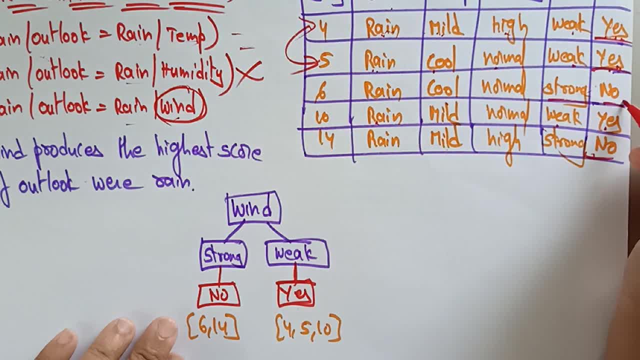 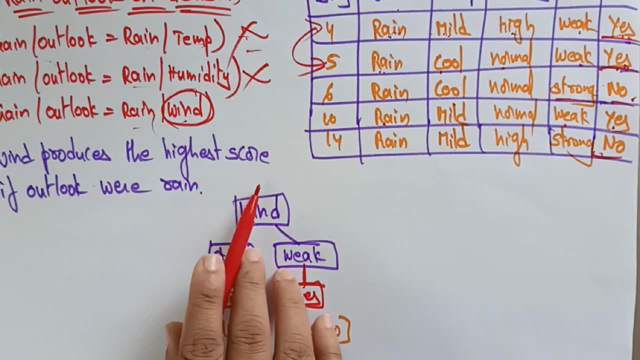 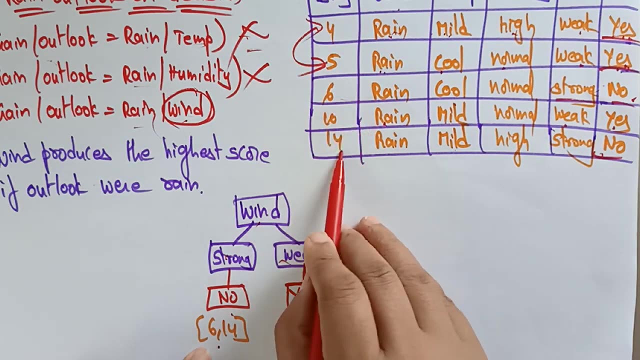 also it is getting. yes, if temperature is cool it is also getting. no means a conflict is arising, so just discard it. only for the wind it is getting matching, so wind produces the highest score. if i rain, so wind is strong, weak and no. so on which days? it is? no, 6 and 14, no, and 4, 5, 6. you can go. 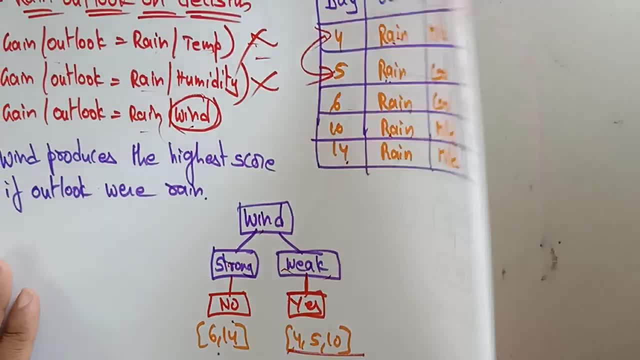 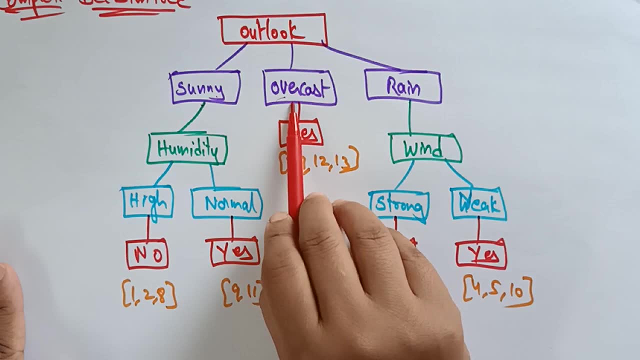 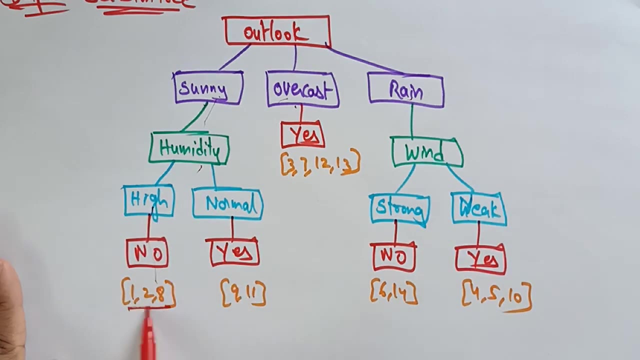 5, 4, 5 and you can go out. so the complete decision tree is like this outlook. so you focus on sunny or overcast rain. so sunny if it is a humidity is there whenever it is high, don't go out in those days. you don't go out. whenever the humidity is normal, you can go out in these days, you can go. 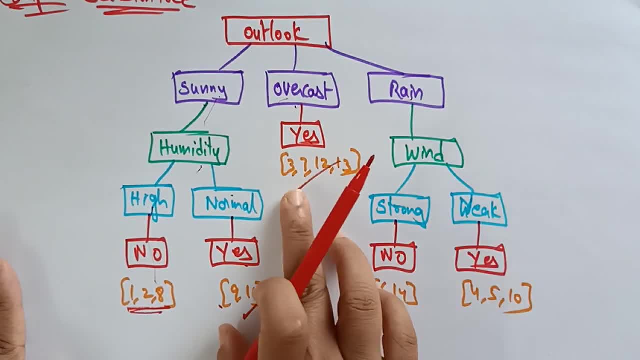 out if the overcast is yes, you can go. in these days, 3, 7, 12, 13 in this- in those days you can go out rain. so whenever the humidity is high, don't go out in those days, you can go out in those days.